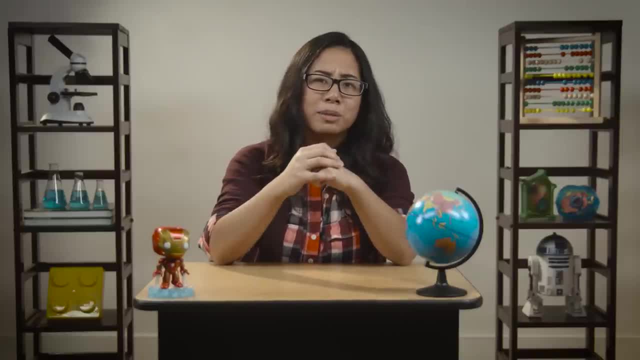 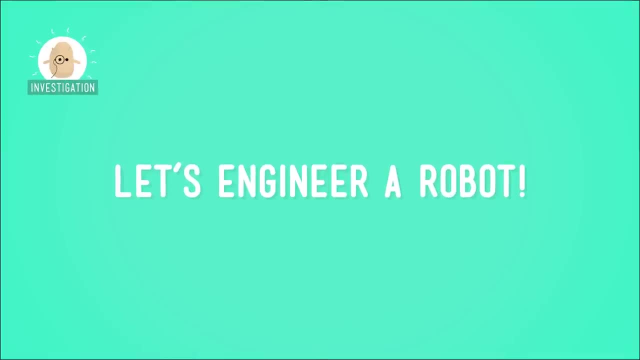 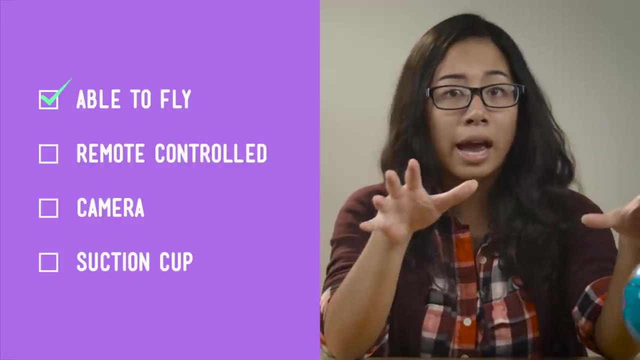 designed for this sort of thing, Not retrieving phones from storm drains, maybe, but flying down into caves, exploring the ocean floor and even visiting other planets. So let's engineer a robot. Hmm, It'll have to be able to fly and be remote controlled And so I can see where it's going. it'll need a little. 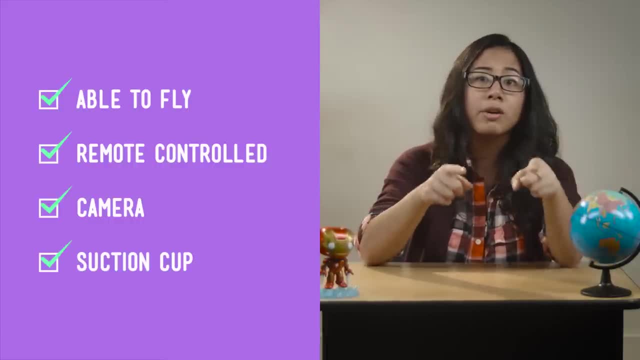 camera And it'll need a suction cup to stick to the phone. And it'll need a suction cup to stick to the phone And carry it to my loving hands Now. next, we need to build a prototype that we can use for testing. 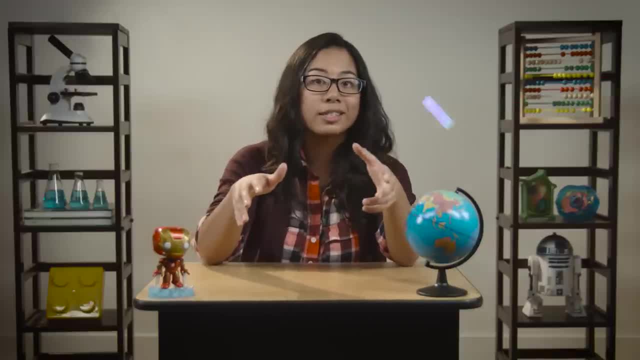 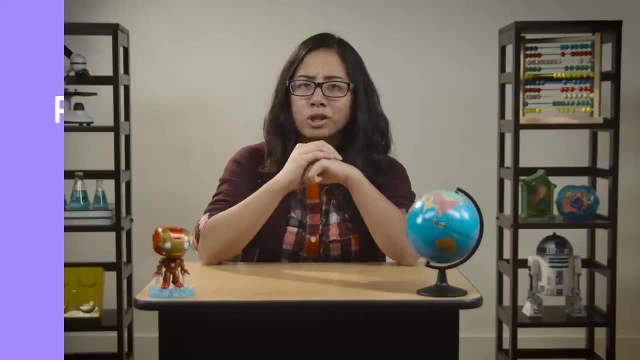 We need to test or conduct trials in order to ensure success. And for those trials to be really useful, we have to isolate the variables. So what are the variables of our mission? We've got the depth of the sewer drain. That can't be. 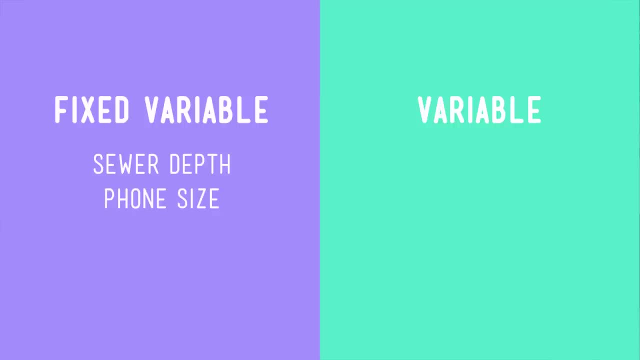 changed, so it's called a fixed variable. We also have the size and weight of the phone, which are more fixed variables. Then we have the pieces of our super cool robot: The propellers, the suction cup, the camera and the. 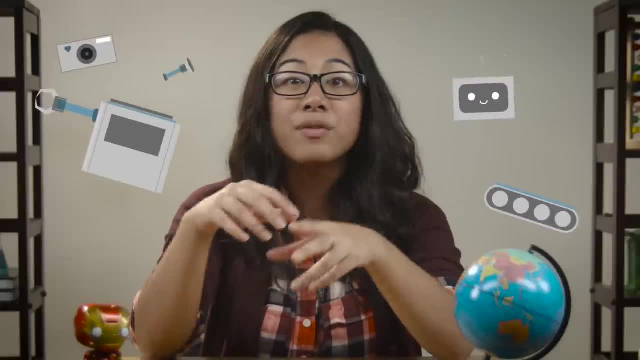 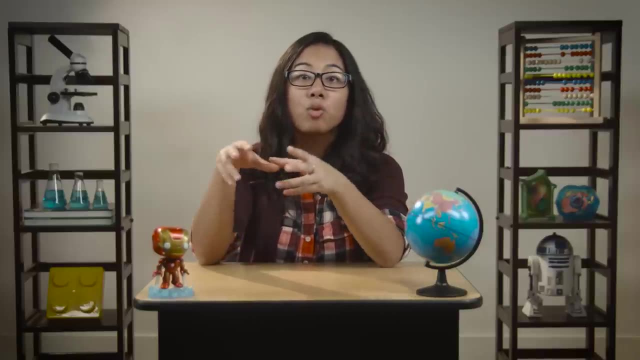 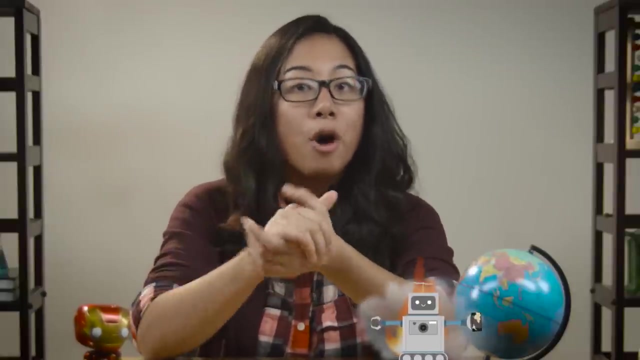 camera. When we finally get to testing the robot, we need to isolate each of these variables and test them one at a time in pretend missions. That way we can see which variables affect how well our robot performs. Like, maybe the robot can carry something the size of a pencil but it completely crashes when it tries to hang onto my phone. That would be a 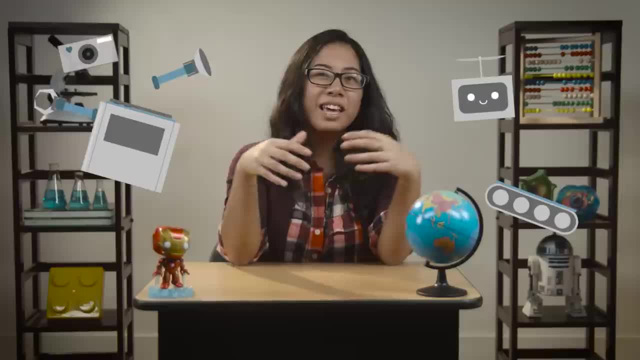 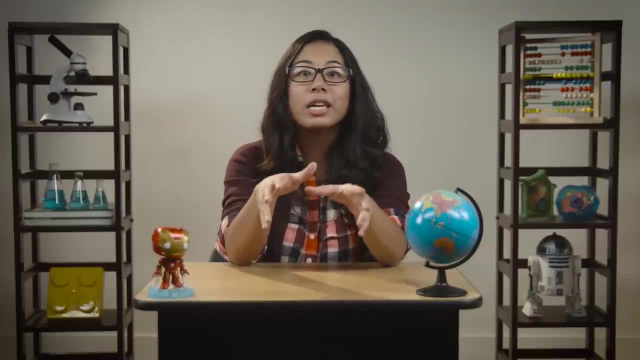 failure point, But we can find ways to science around that. If it can't lift something as heavy as my phone, maybe we can make the propellers bigger. Either way, we'll keep tweaking the variables until we get the outcome we're looking for. Then it's all: systems go Hang on. wet and smelly phone, Here we come. 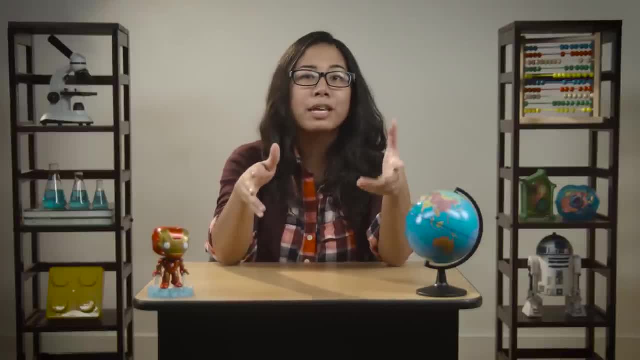 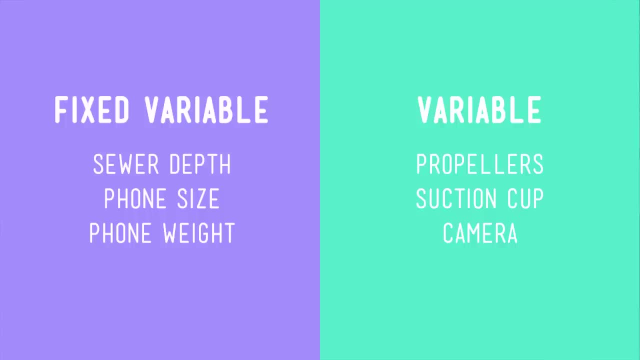 Today we had a challenge. We had to retrieve something from a deep place we couldn't see, And we had to deal with various variables to find a solution. Variables like the depth of the drain, the weight of the phone and the strength of the. 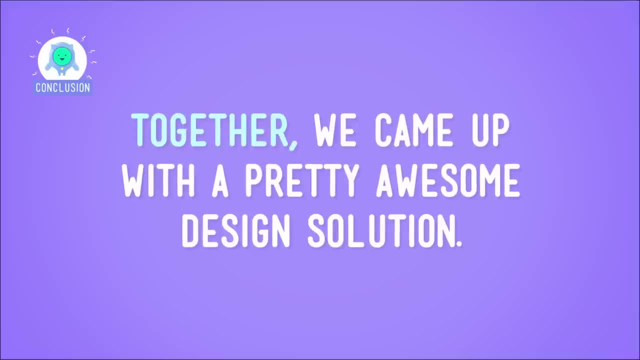 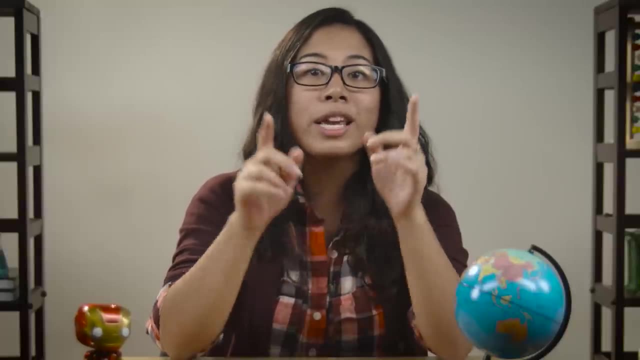 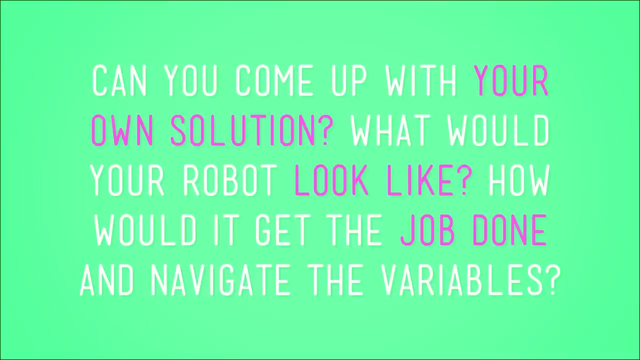 propellers that made the robot fly. Together, we came up with a pretty awesome design solution, But, like I said before, there can be lots of different success stories. So here's your challenge: Can you come up with your own solution? What would your robot look like? How would it get the job done and navigate the variables? 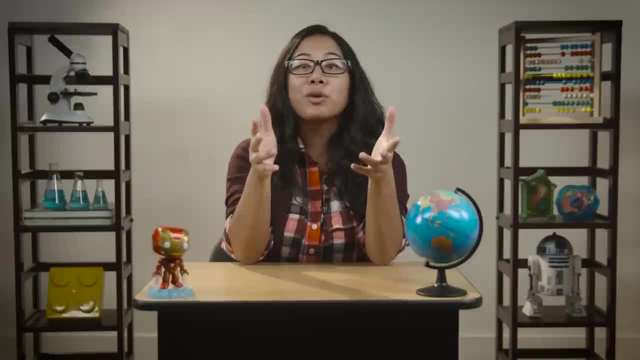 Put your brain to work and see what you can come up with. As for me, this isn't the first jam that engineering helped me to get out of, And I'm sure it won't be the last.